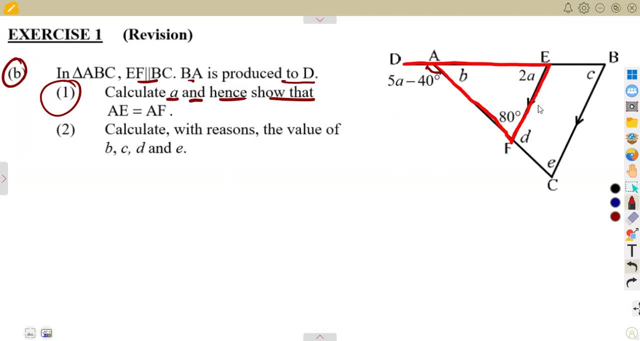 So it's a triangle, this one. There is an angle of 2A, There is an angle of 2B, There is an angle of 80.. There is 5A minus 40.. 5A minus 40, this angle is the exterior angle of the triangle. 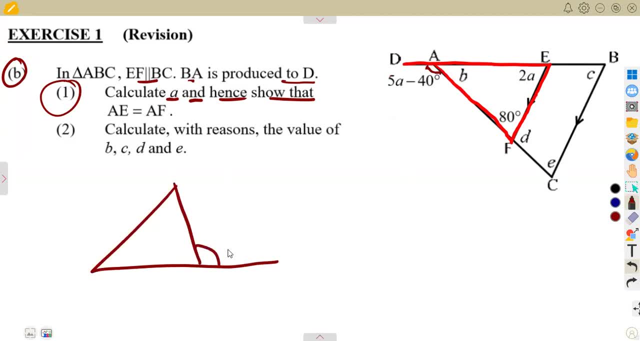 And remember that it is always that The exterior angle is equal to the sum of the opposite interior. If there is A and B, if you add these two, they are supposed to give you the exterior. This is the concept, the exterior angle, this one of 5A. 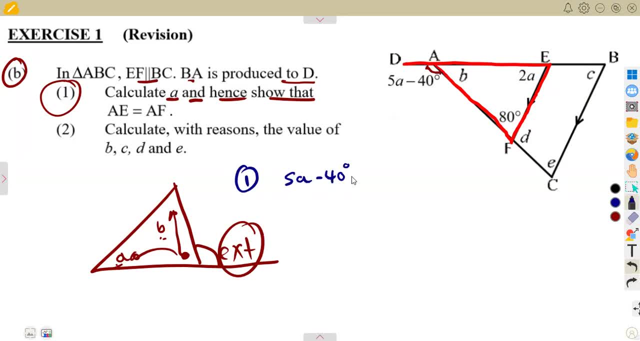 The exterior angle of 5A minus 40 degrees is equal to what? Because that's our exterior angle. It must be equal to the sum of the what, The opposite interior, the 2A and the 80 degrees, The ones that are opposite to this interior angle, which is the 2A and the 80 degrees. 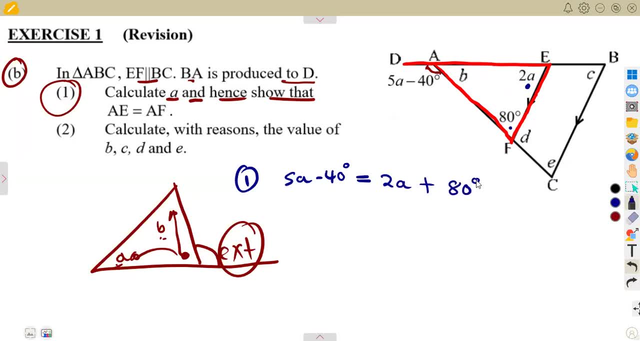 So that's 2A plus 80 degrees. So it's an equation. So exterior angle is equal to what Sum of what Opposite interior angles? That's the concept. So we can solve for A from this equation, All right. 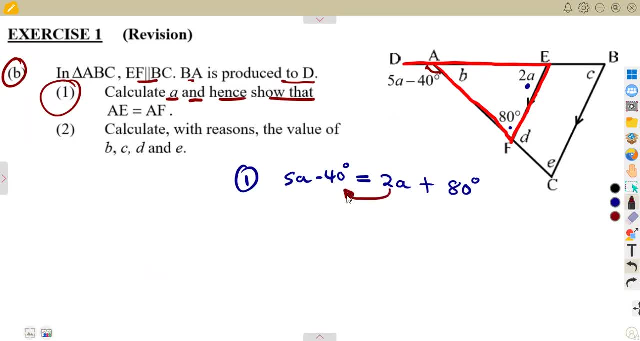 So collecting the terms of A to one side of the equation, this is going to be 5A, So 2A- on this side it will be minus 2A- is equal to transpose the minus 40 on the other side of the equation. 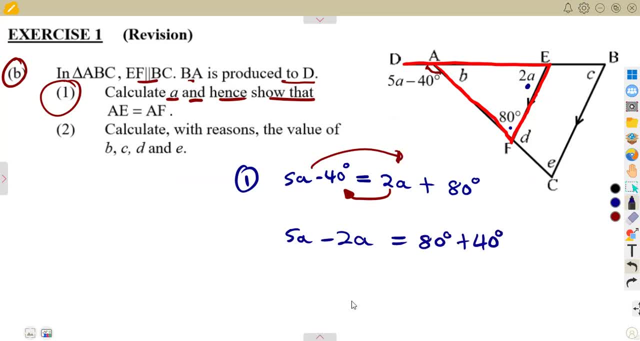 That will be a plus, So it's 80.. Plus 40 degrees, 5A minus 2A, that is going to give us 3A, which is equal to 40 and 80 together, That is going to give us 120 degrees. 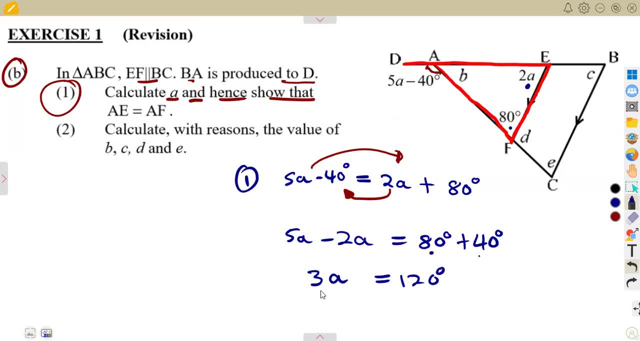 Remember that this is an equation, So you can solve for A, just like our normal linear equation. So you can divide by 3 because you are multiplying. So divide by 3 both sides. Our A is going to be what 120 divided by 3.. 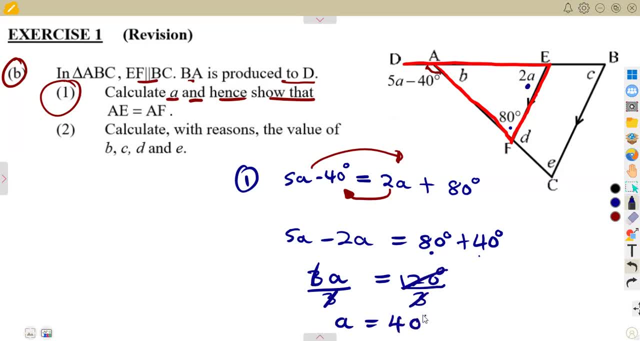 That is 3 into 120 from your calculator, You are going to obtain a 40 degrees. So this is the value of A which satisfies this condition. Yens show that AE is equal to AF. How can we show that AE is equal to AF? 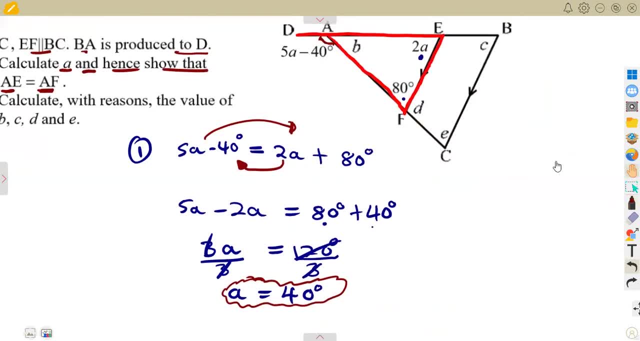 We simply need the angles. We know that if the two angles are equal, If these two angles are equal, the sides which are opposite these angles are also equal. So is that the case? Okay, we calculated, our A is 40.. All right angle AEF. 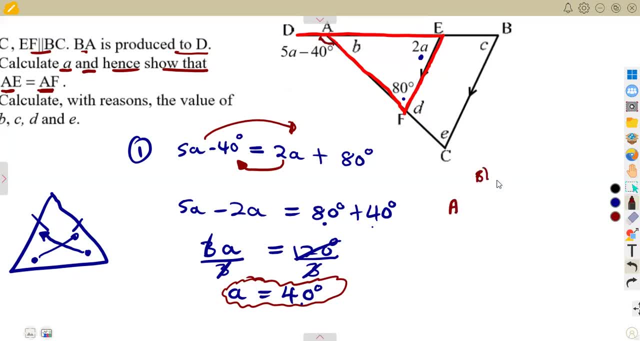 It follows that This is now to show that the part of what, of showing that show that this is AEF, Is to a, which means two times angle: a, which is 40 degrees and that is 80 degrees, Meaning to say, if a is 40 degrees, this angle that we are seeing here is 80 degrees. 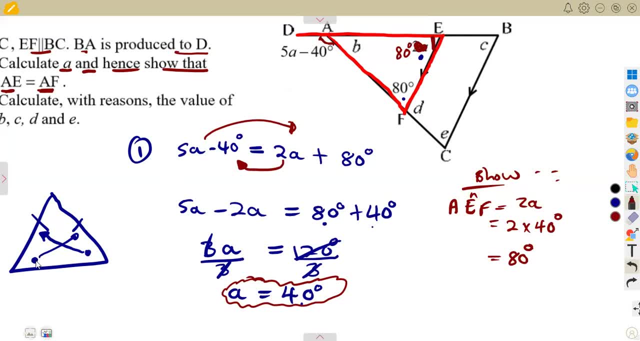 That is what we have, And this is exactly the consideration that we have. If these two angles are equal, the sides which are opposite, opposite these Angles are equal. So, therefore, AE is equal to what to AF? All right, So these are sides. 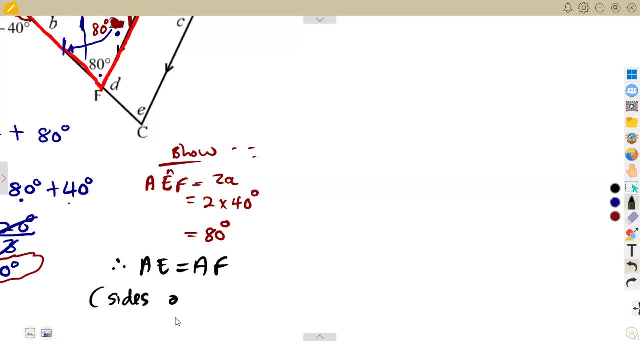 We are talking about what sides Opposite Equal angles. All right, They are supposed to be equal. also, Whenever you see this happening is the same, So it can be from the sides. If you are given sides which are equal, it also follows that the angles that are opposite those sides- they are supposed to be equal. 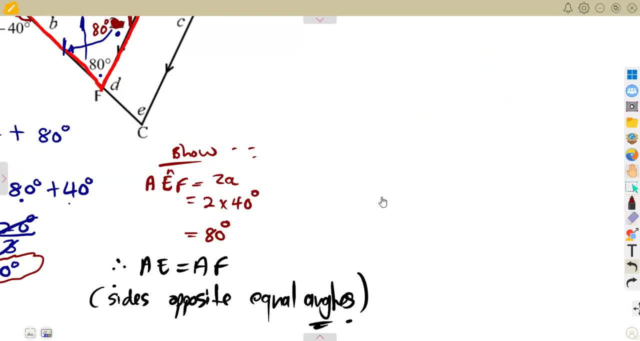 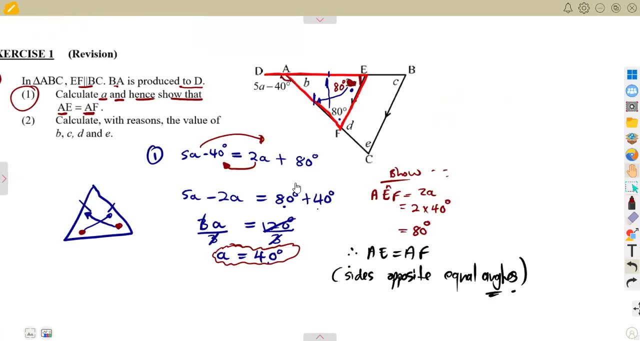 So it depends with what are you given? Are you given as equal angles? You prove that the sides are the same. Are you given as the sides? That is the idea. Calculate with reasons the size of the angles B, C, D and E. 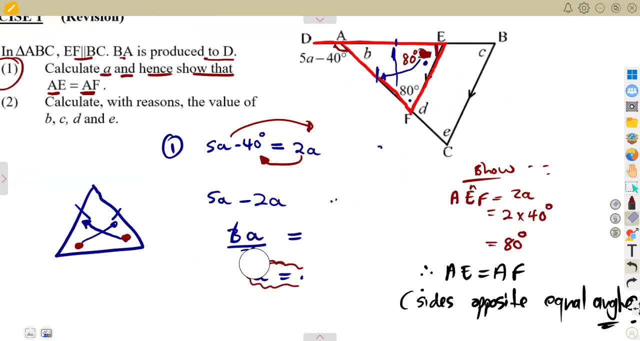 All right, Already we calculated our angle A, So it's just going to be a continuation from that, using our theorems, working with our parallel lines, the shapes, angles in a triangle, and so forth. All right, So let us check what we have. 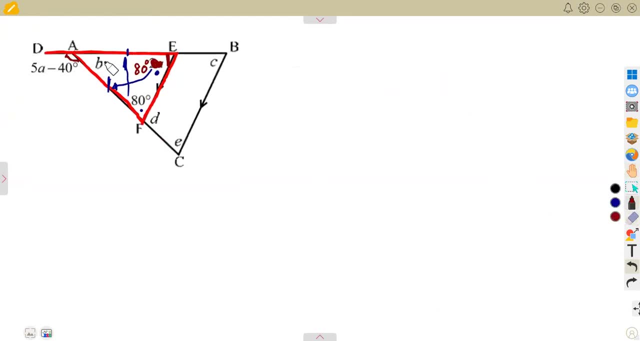 We can calculate angle B if we are to consider these angles in a triangle, or you can consider angles on a straight line. It's up to you. So angle B, that is 180 degrees minus the 80. And the 80 using angles in a triangle. 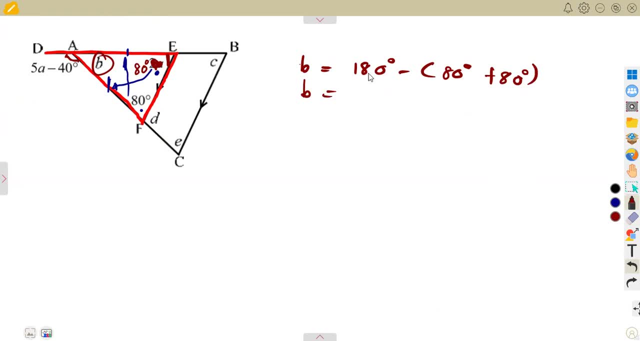 Remember that angles in a triangle, they add up to 180 degrees. That's 180 degrees, All right. So meaning to say that was going to be 160, 180 minus 160 is 20 degrees. So there we are talking about angles in a what? 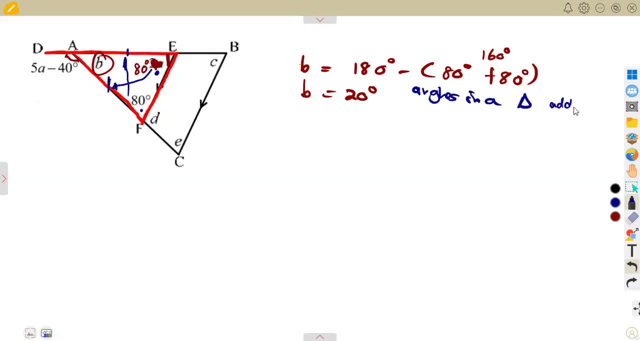 Angles in a triangle add up to 180 degrees. They add up to 180.. Or maybe you substitute your A here. Then you can use angles on a straight line. That one is up to you, All right. So we have got our angle B, which is 20 degrees here. 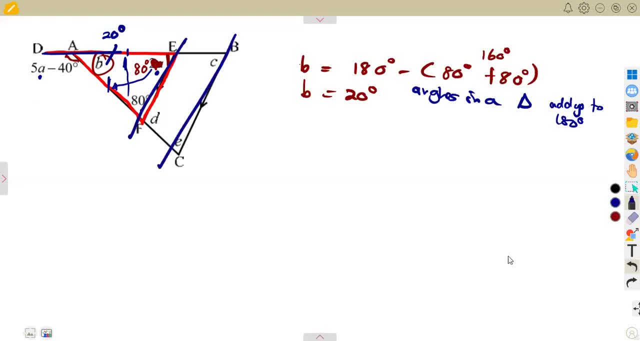 All right. What about angle C? These two lines, they are parallel. These two lines are parallel. So it follows that wherever you create an F like this, these are corresponding angles. And I said corresponding angles are equal. So if you are to check properly, 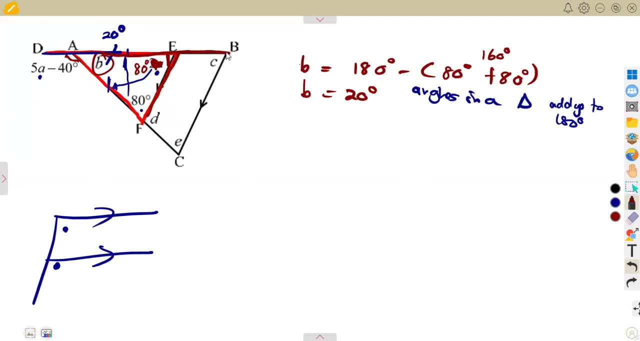 We are creating an F this way. even though it's like this, that's an F, That one, the way that it is like this, this angle and this angle are equal, So it also follows that angle C is equal to 80 degrees. 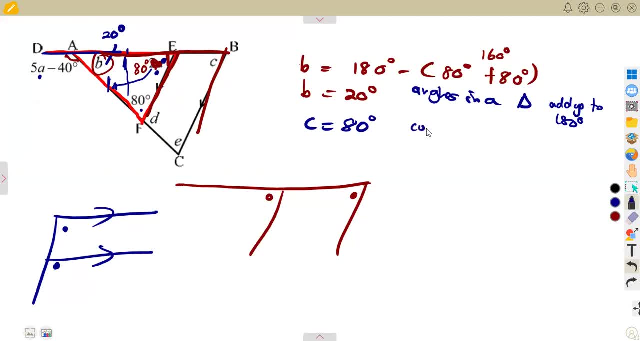 That is 80 degrees, This one. So this is from corresponding angles. All right, Remember, corresponding angles are equal. Okay, The same thing with angle E. So this is: This is 80 degrees, The same with angle E. 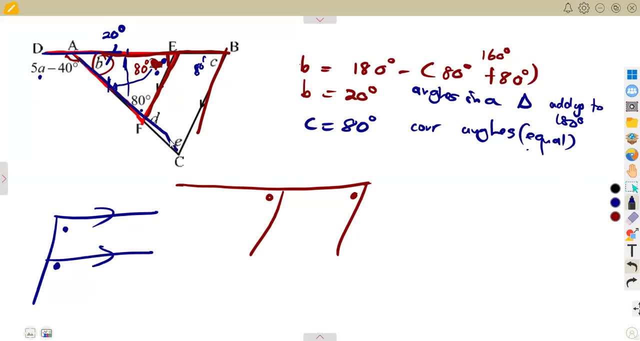 This is corresponding from this side. If you check, this is an F which is drawn this way. All right, This is an F which is drawn this way. So this angle and this angle are also equal corresponding angles. We are still having the corresponding angle concept.